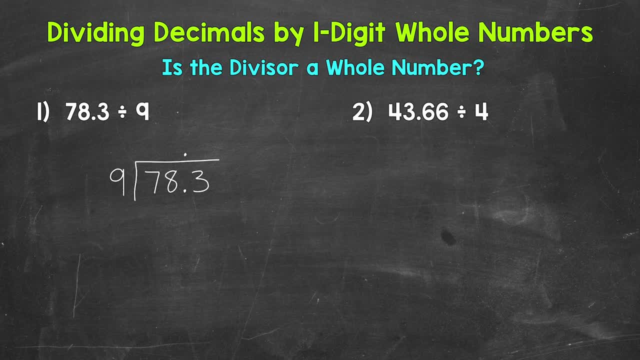 If yes, bring the decimal straight up. Now we go through our division process, The same exact process we use when we divide whole numbers. So divide, multiply, subtract, bring down, repeat. Let's start with divide. So we have 7 divided by 9.. 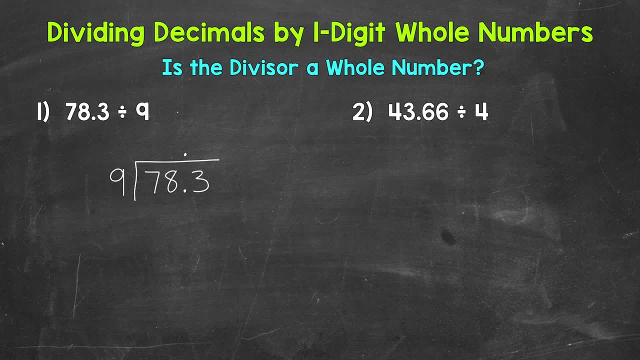 How many whole groups, How many whole groups of 9 in 7?? Well, we can't do that, So we need to look at the 7 and the 8. So we have 78 divided by 9.. How many whole groups of 9 in 78?? 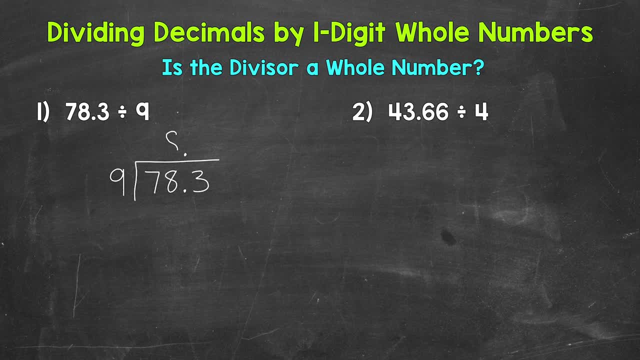 Well, 8. That gets us to 72.. Make sure to put the 8 above the 8 in 78,, not above the 7. We used both the 7 and 8 and did 78 divided by 9.. 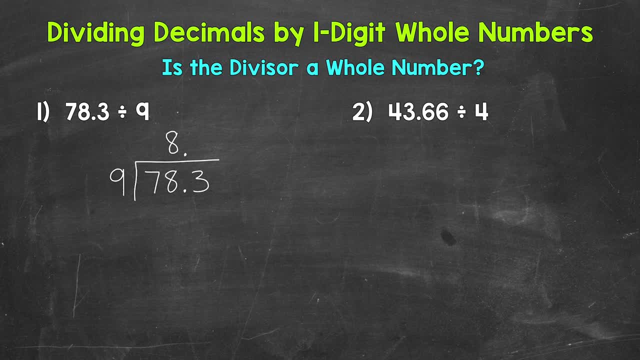 So again that 8 needs to go above. So we need to look at the 7 and the 8.. Now we multiply 8 times 9, 72,. subtract 78 minus 72 is 6, bring down now we have 63. 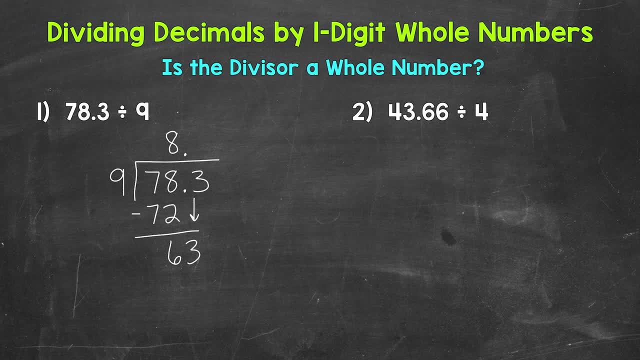 And we repeat. so we go back to divide: 63 divided by 9. How many whole groups of 9 in 63?? Well, 7. And that hits 63, exactly 7 times 9.. 63. Subtract. 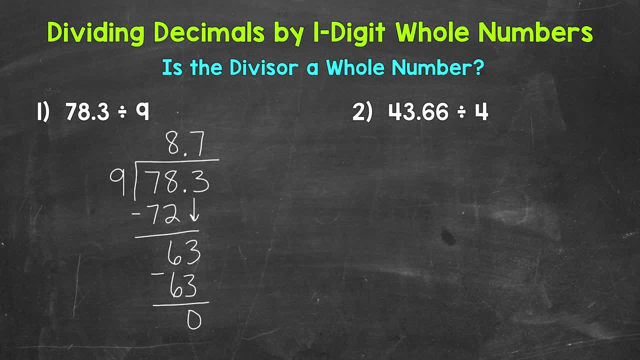 63 minus 63 is 0.. We went all the way over to the furthest place to the right, which was the tenths place for this problem, And we have a clean cut 0 here at the end. So we are done. 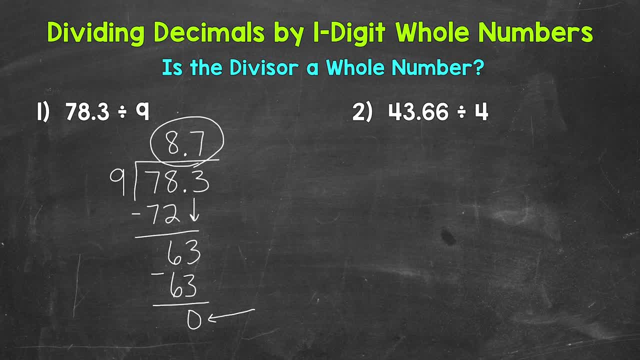 8 and 7 tenths. Now for number 2, we're going to see what happens when we don't get that clean cut 0 at the end, And we need to extend the problem until we do And we do get that clean cut 0. 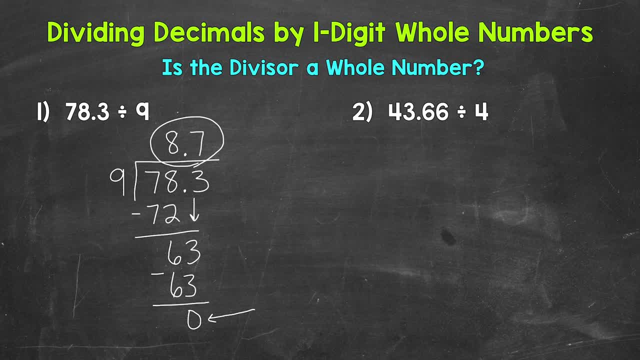 Let's move on to number 2, where we have 43 and 66 hundredths divided by 4.. We will start by setting this problem up, And I'm going to come to the side here, because this one will need a little more room than number 1 did. 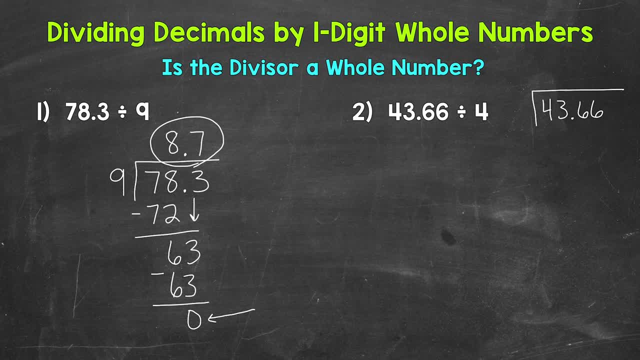 So 43 and 66 hundredths is the dividend, the number we are dividing. We are dividing by 4.. That is the divisor, the number we are dividing. Is the divisor a whole number? Yes, So bring the decimal straight up into the answer. 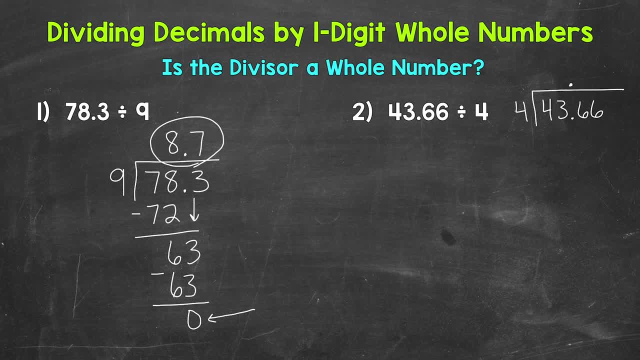 Now we go through our division process. Start with divide. So we have 4 divided by 4. How many whole groups of 4 in 4? 1. Now we multiply 1 times 4.. 4. 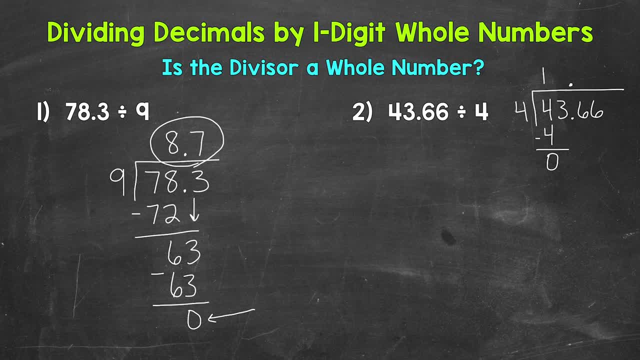 Subtract 4 minus 4.. 0. Now we bring down, So we have 3. And we repeat, So we go back to divide 3 divided by 4.. How many whole groups of 4 in 3?? 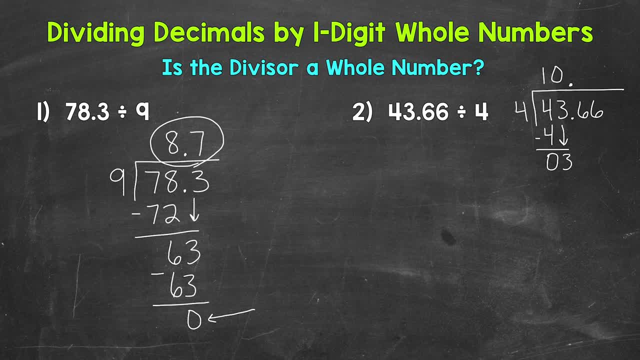 Well, we can't do that, So we need a 0. Now we multiply 0 times 4.. 0. Subtract 3 minus 0. 3. Bring down Now: we have 36.. 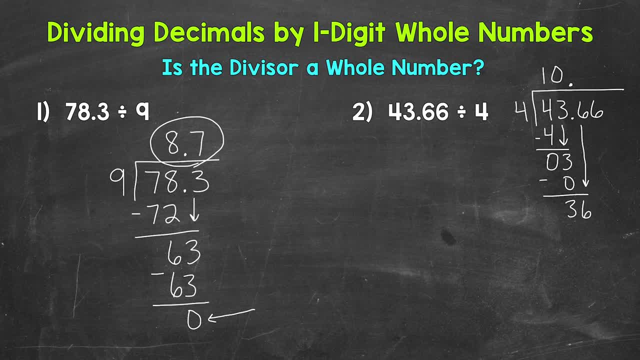 And we repeat So: divide 36 divided by 4. How many whole groups of 4 in 36? 9. That hits 36 exactly. Multiply 9 times 4.. 36.. Subtract 36 minus 36 is 0.. 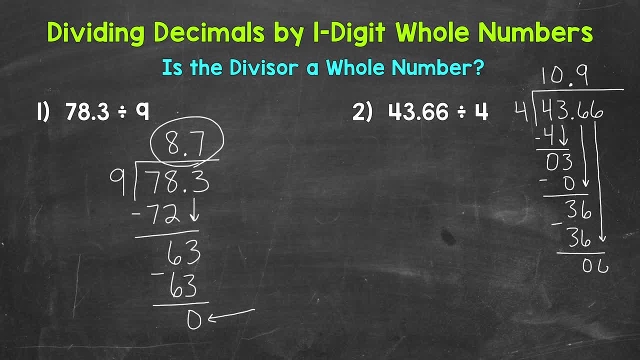 And then bring down: That's 6.. We have 6 there And we repeat: So go back to divide: 6 divided by 4.. How many whole groups of 4 in 6?? 1. Multiply 1 times 4.. 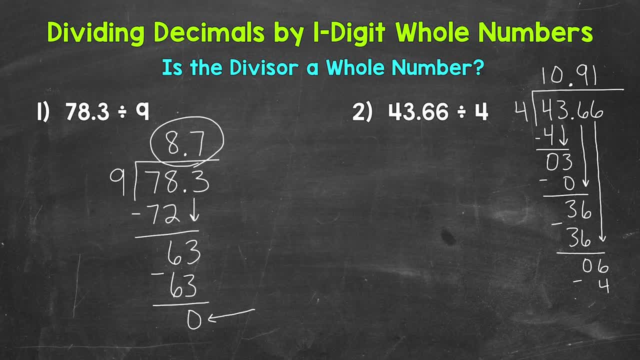 4. 4. Subtract 6 minus 4 is 2.. We went all the way over to the furthest place, to the right, The hundredths place, But we have a 2 at the end. We do not have a clean cut 0 yet. 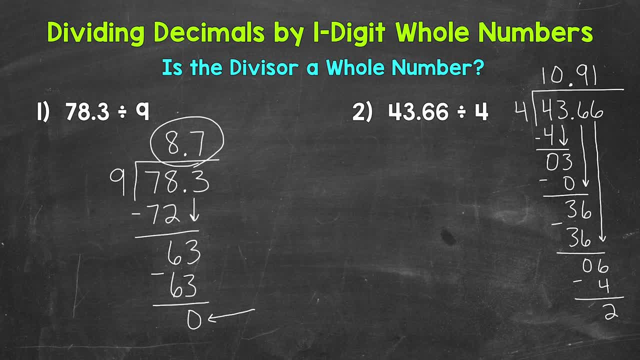 That 2 does not mean remainder 2, like when we work with whole numbers. This answer is in decimal form, So we need to keep it that way. What we can do is extend This problem until we do get a clean cut: 0..